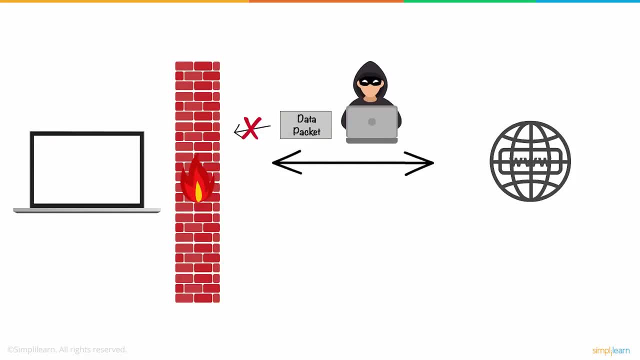 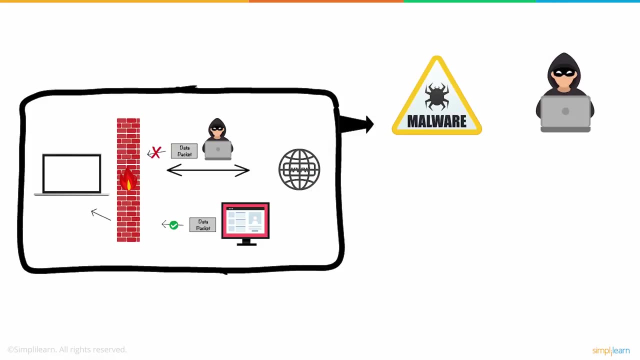 and the internet. The firewall rejects the malicious data packet and thus protects your network from hackers. On the other hand, traffic from trusted websites is allowed access to your network. This way, the firewall carries out quick assessments to detect malware and other suspicious activities, thereby protecting your network from being susceptible to transactions. 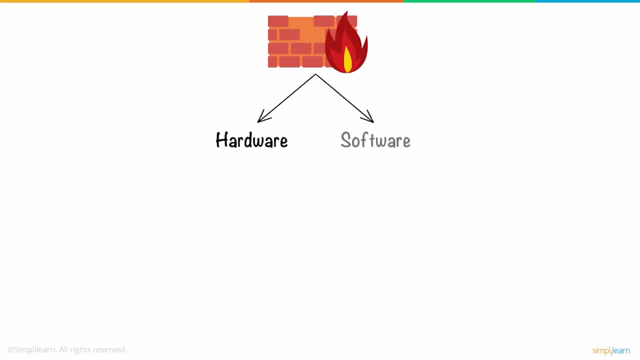 a cyber attack. Firewalls can either be hardware or software. Software firewalls are programs installed on each computer. This is also called a host firewall. Meanwhile, hardware firewalls are equipments that are established between the gateway and your network. Linksys routers are a. 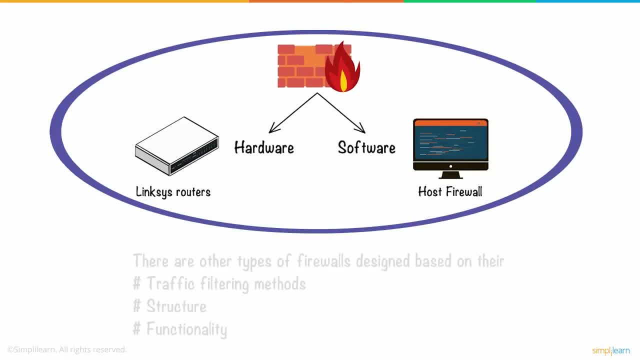 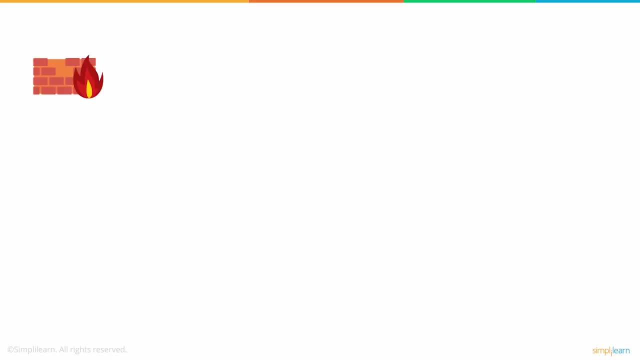 good example of a hardware firewall. Besides this, there are other types of firewalls designed based on their traffic filtering methods, structure and functionality. The firewall that compares each outgoing and incoming network packet to a set of established rules, such as the allowed IP. 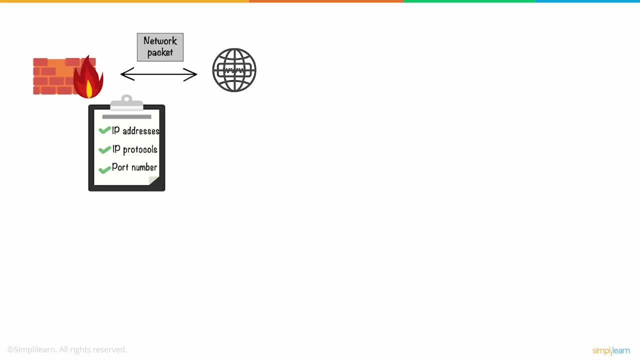 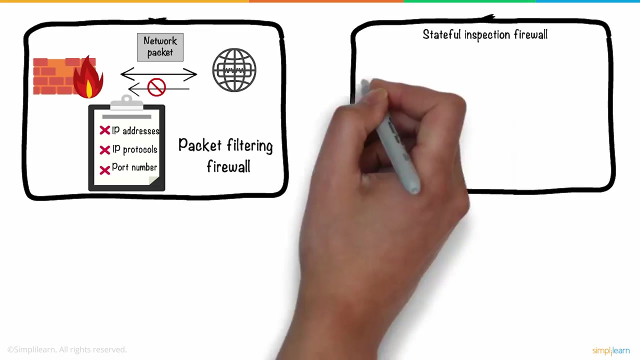 addresses, IP protocols, port number and other aspects of the packet is known as a packet filtering firewall. If the incoming network traffic is not per the predefined rules, that traffic is blocked. A variant of the packet filtering firewall is the stateful inspection firewall. These types 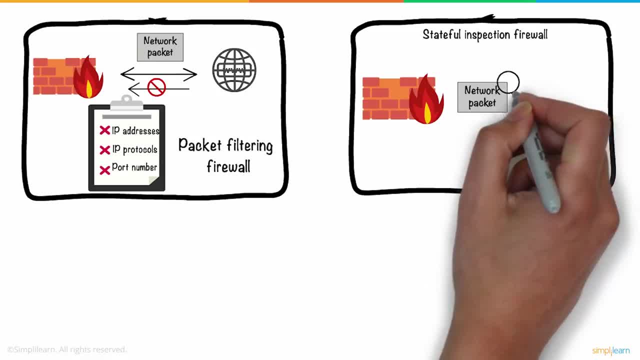 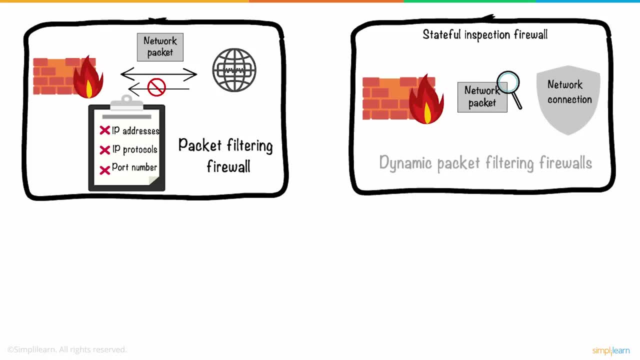 of firewalls not only examine each network packet, but also checks whether or not that network packet is part of an established network Connection. Such firewalls are also referred to as dynamic packet filtering firewalls. Our next type of firewall is called a proxy firewall. This draws close comparison to how you give proxy attendance. 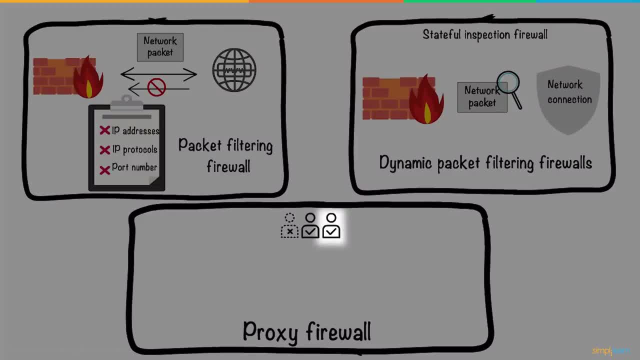 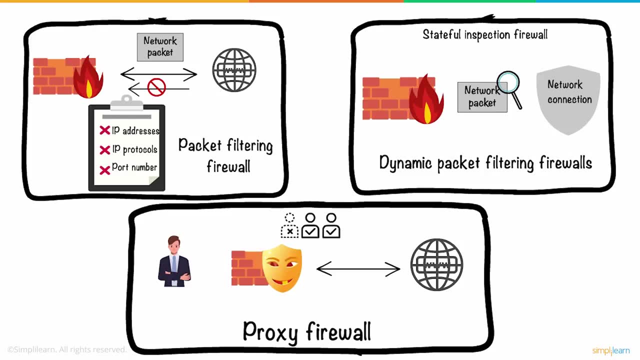 for a friend, like how you take the authority to represent your friend. The proxy firewall pretends to be you and interacts with the internet. They come between you and the internet and thereby prevents direct connections. This protects your device's identity and keeps the network safe from. 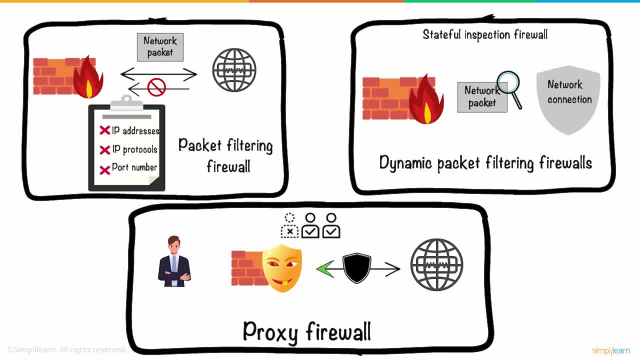 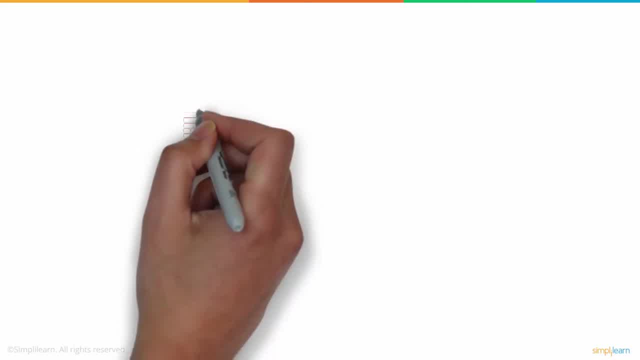 potential attacks. If you have an internet connection problem, you can use a proxy firewall to prevent potential attacks. Only if the incoming data packet contents are protected, the proxy firewall transfers it to you. They are also known as application-level gateway. A firewall can spot. 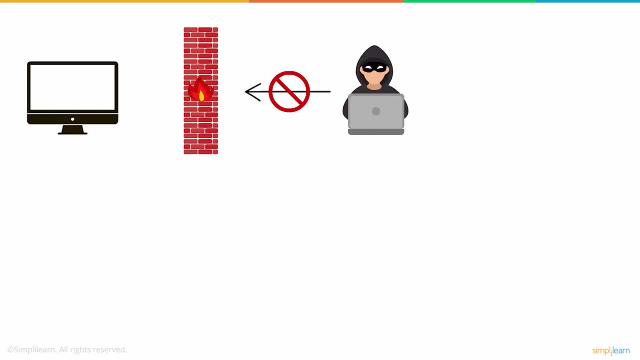 malicious actions and block your computer from receiving data packets from harmful sources. In addition to preventing cyber attacks, firewalls are also used in educational institutions and offices to restrict users' access to certain websites or applications. It is used to avoid access to unauthorized content, So if you have an internet connection problem, you can use a proxy.